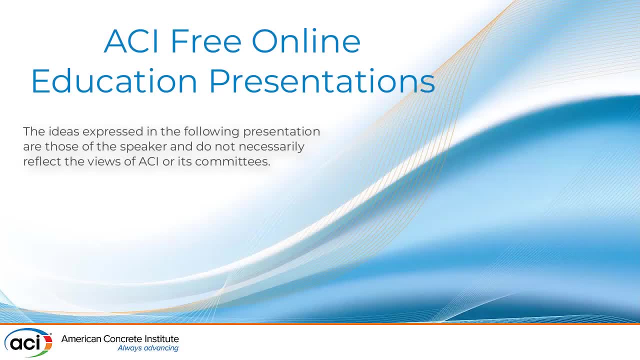 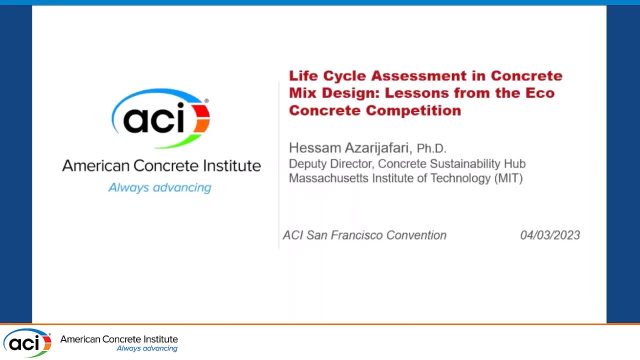 Thank you very much for the introduction and for inviting me for this session. Hi everyone, my name is Hesam and I'm working as Deputy Director of the MIT Concrete Sustainability Hub. Today, I'm going to share some of the lessons that we learned from the ACI Eco-Concrete. 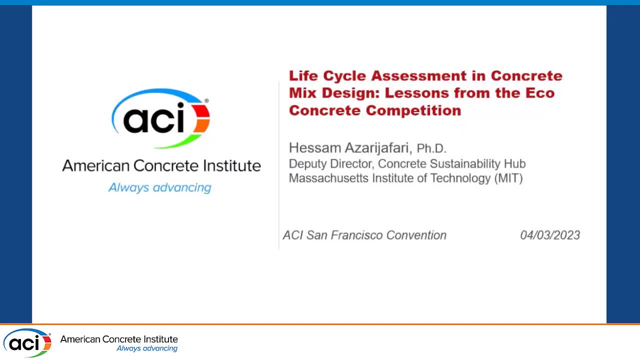 Competition. Believe it or not, we've been holding this competition since 2017, when I was a PhD student at the University of Sherbrooke. We put together the rules and a small tool to quantify the environmental impacts, and then we had this analysis and shared with. 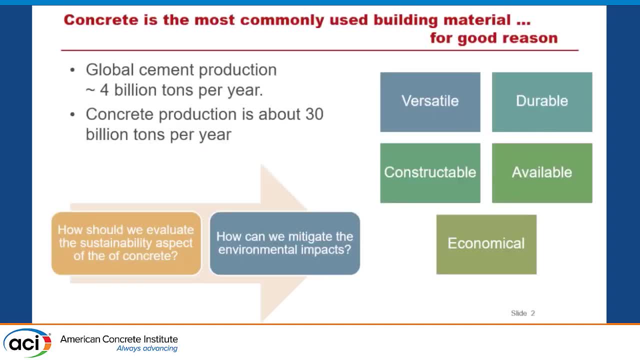 the students as well. So, again, why is it important to consider concrete? We are facing this versatile, constructible, durable, sustainable, sustainable, sustainable, sustainable, sustainable, economical and available materials around the world, and everyone is using that for urbanization. 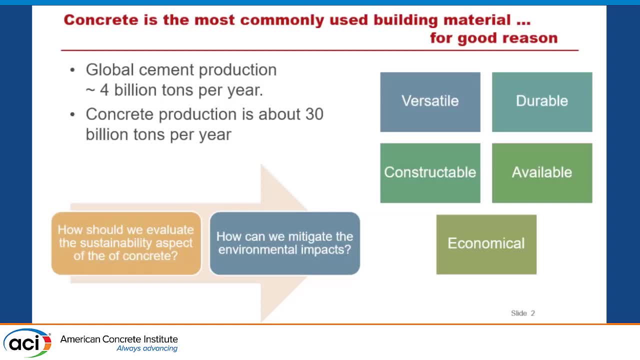 and we are going to use that in the future more and more because of the population growth and our demand in the future And because of all these benefits. this is part of our daily construction, but we have to think about this huge amount of materials- more than four. 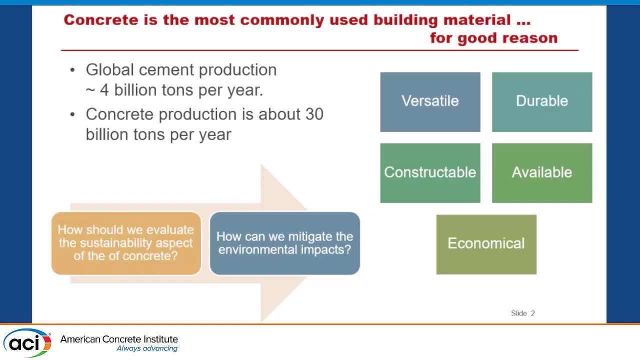 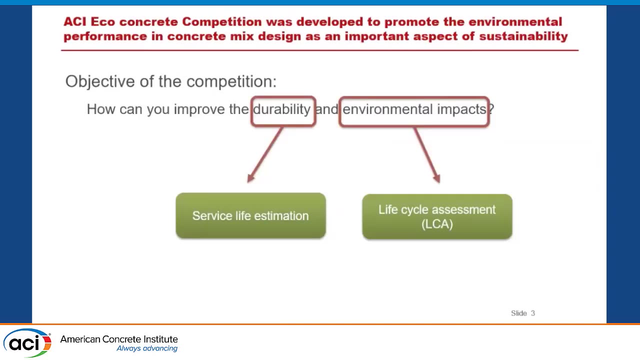 billion tons of cement and maybe 30 billion tons of concrete per year is produced around the world and we have to think about how to reduce the environmental impacts of these concrete mixtures. And the idea of Eco-Concrete comes from this important research question and we put together the main objective as to promote the environmental impact as an 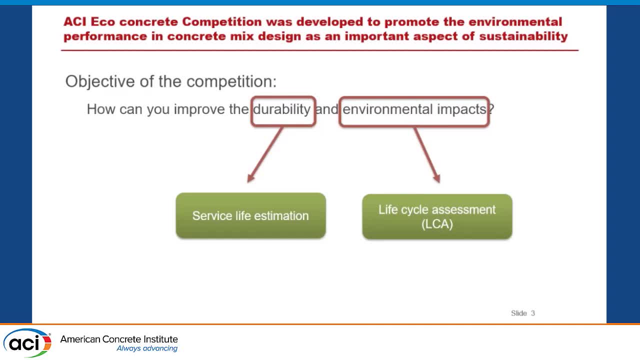 important part of the sustainability of concrete. with regards to the performance, Many other sustainability evaluations do not usually usually consider the performance, but we as engineers know that it's important to consider and make the decision with regards to what we call here as performance, And it could. 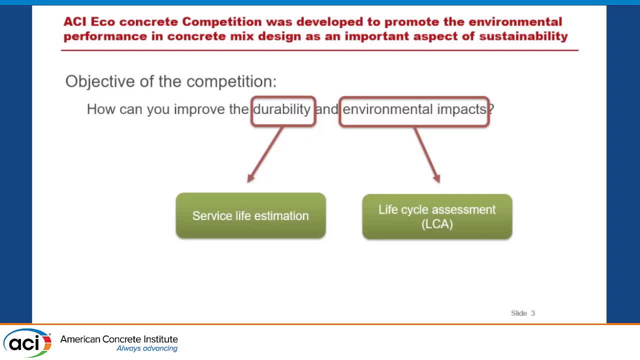 be defined in different ways. We have hardened performance, including the mechanical durability properties, aesthetic purposes or aesthetic functionality. These are all different aspects that we can include, But in this competition, in addition to the environmental assessment, which was conducted through life cycle assessment, we considered durability as the main mechanism. 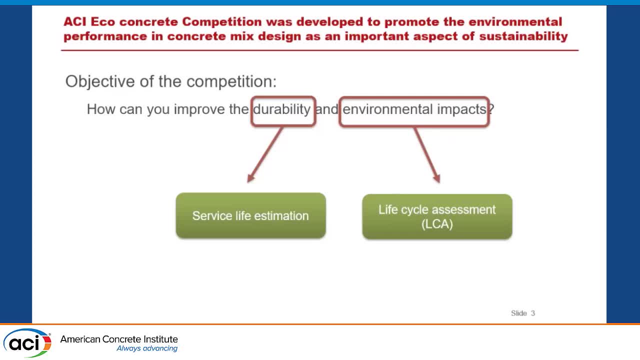 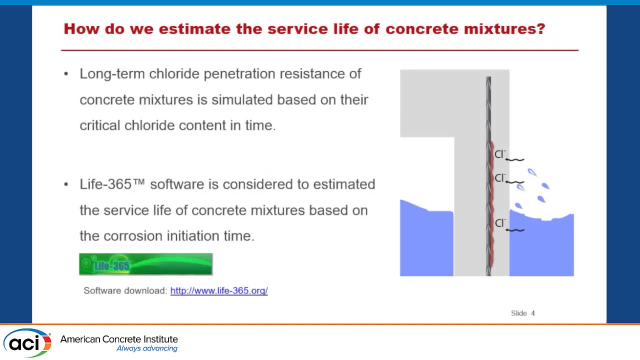 and determining factors for the performance of the mixtures. And for that, For this competition, we asked these questions that how can we estimate and improve the service life of concrete performance when it's exposed to the aggressive environment? And for that purpose we used this Life 365 tool to enable the students to quantify the service life. 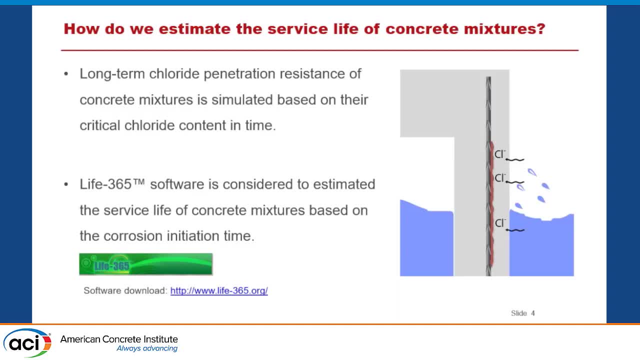 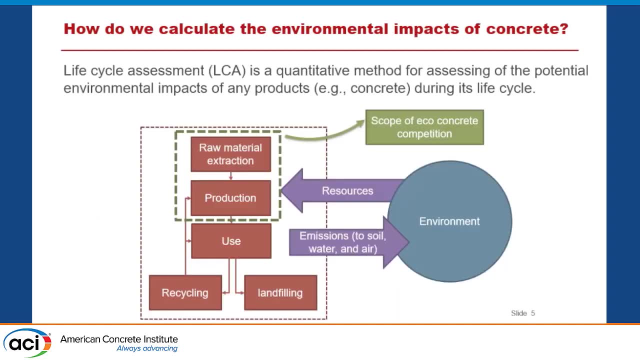 of the concrete, given a specific exposed conditions and concrete dimensions as well. This is about the performance for life cycle assessment. As you probably know, it's a quantitative method that will help us quantify the environmental impacts of any products or services, including concrete mixtures, And it assesses the environmental impacts from very early stage of the production. 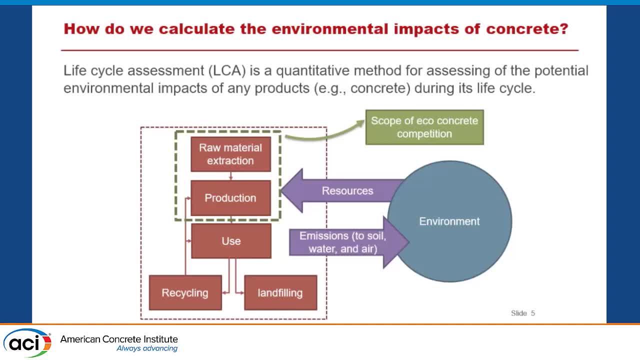 raw material extraction, Then we consider the production, Then we consider the material extraction, use and end of life, whether we recycle, reuse or landfill that product. So cradle to grave scope. But for the purpose of this competition we definitely focused. 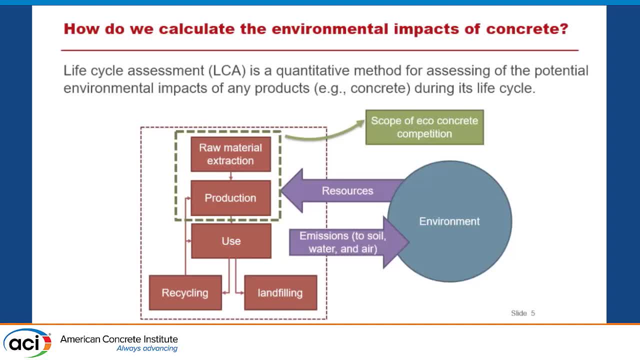 on the raw material extraction and production of the materials. for the sake of simplicity and assuming that during the use and end of life we have equal performance in terms of the environmental impacts, What did we ask from the students? We asked them to design two different mixtures. 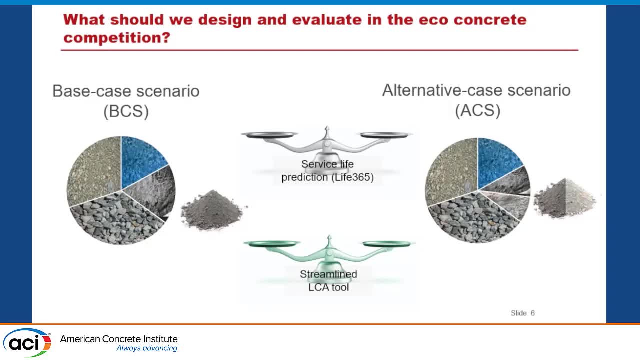 This case scenario- here I just use this abbreviation BCS- And the other one is alternative case scenario ACS. In the base case scenario they consider regular ordinary Portland cement plus virgin aggregates and water- tap water- for their mix design And in their alternative. 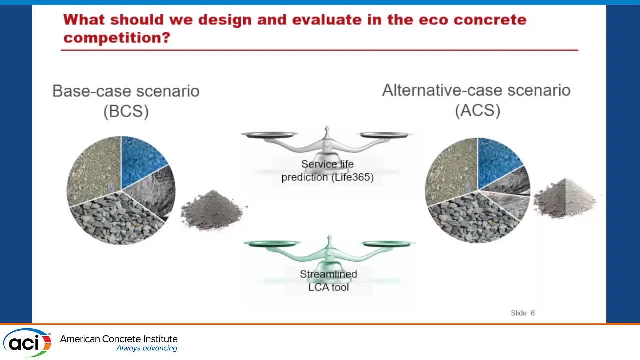 case they have to maximize the amount of environmental benefits while thinking about the durability as the performance factor. So it's a kind of trade-off And we gave different weights to these two different mix designs And we are going to measure their difference based on the streamlined LCA tool that we developed and I will show. 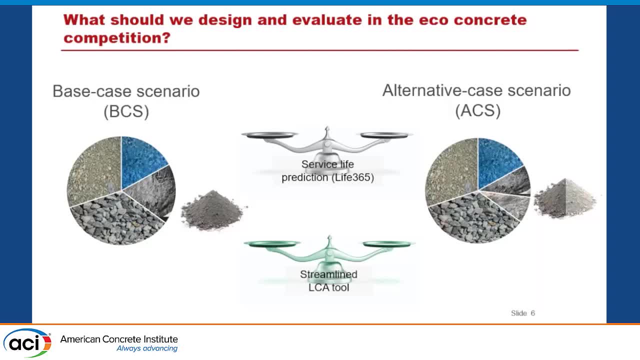 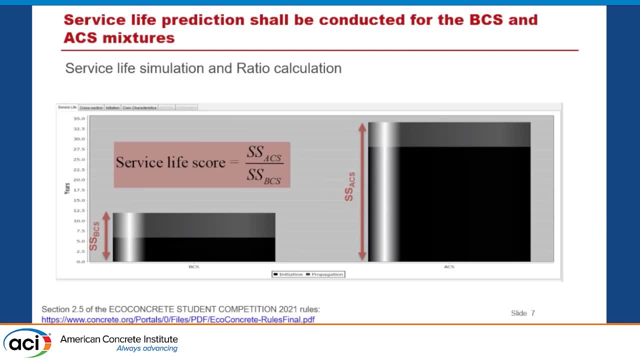 you and also the service life prediction using LIFE 365. And for the service life simulation, like I said, it's LIFE 365. And you have different ingredients prescribed already and included in LIFE 365. And it enables the students to choose different proportions and different components: binary, ternary and quaternary. 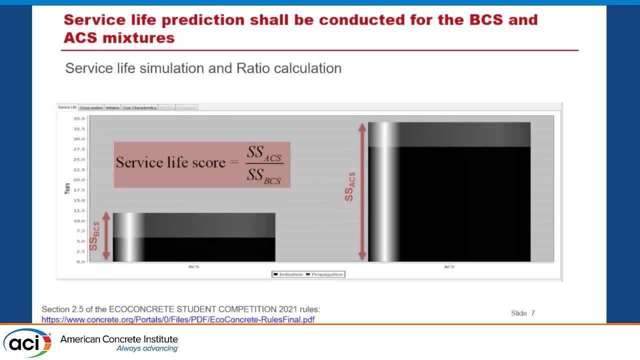 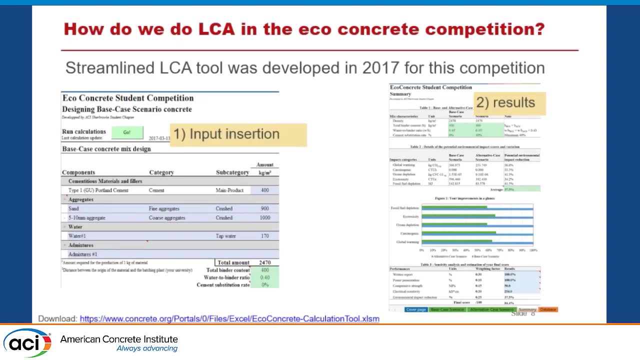 mixture to achieve the maximum performance in terms of the service life extension. How did we do the LCA? We, just When I was a PhD student, we developed an ACI student chapter at the University of Sherbrooke. We created this Excel-based tool. It's available. 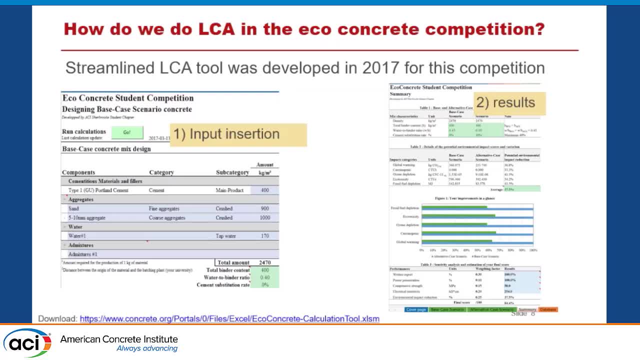 on the ACI website. Feel free to download and play with that. It's available on the ACI website. So I've just shown you how to do this. Here we have another feature. I've just made a new application Here. we have a new component. Here you can see the material. 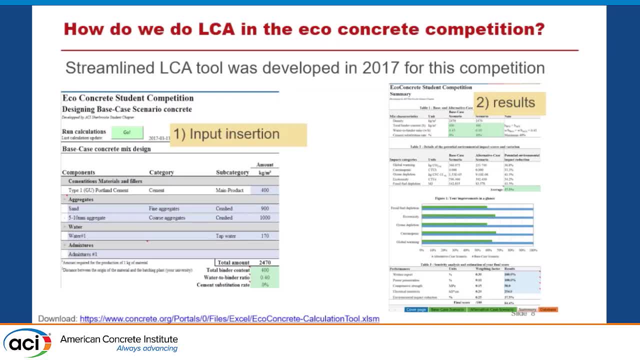 that for educational purposes. obviously, Here you have two different, two main worksheets. One is the inputs, where you enter the type and quantity of the materials that you use for the mix design, and the second one is where you see the final results and there are some color codes over there that will show. 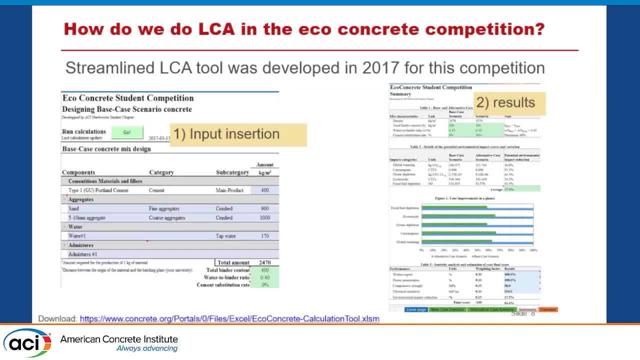 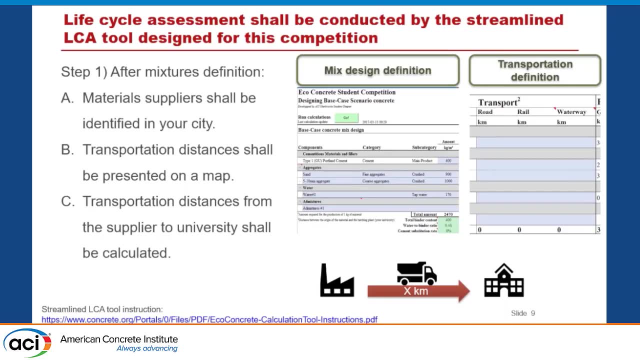 you if you have followed the rules and if there is any conflicts with the rules as well. The other important aspects of this tool when you are going through the cradle-to-gate lifecycle assessments here for concrete mixture, is to define your material supplier sources, because it's very important for us that students 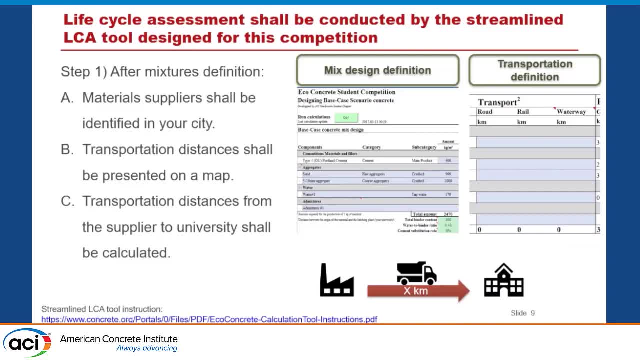 consider the transportation distance and the associated emissions between the source of the materials and the ready mix, plant that for the sake of this computer. In addition, we consider the university, so we want them to definitely consider whether the materials is imported for another from another country, or whether 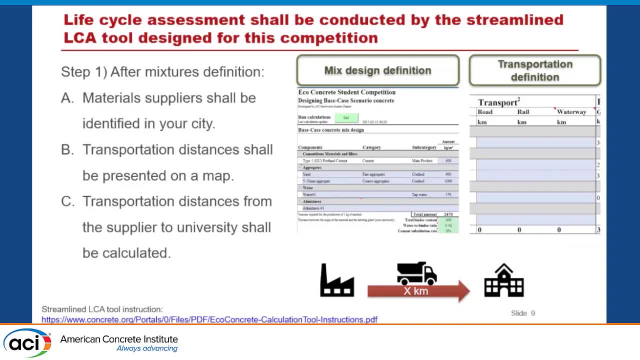 it's locally produced and what's the associated environmental impacts. Again, the objective is to give them this holistic approach and let them think about not only the transportation distance from the local distributor but, very, you know, initial source of production. For example, in many countries, from this competition we realize that they don't have locally. 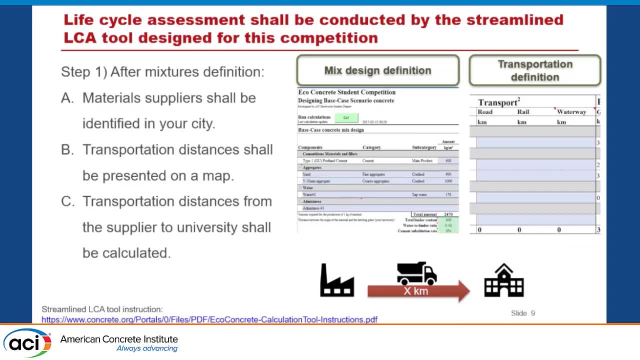 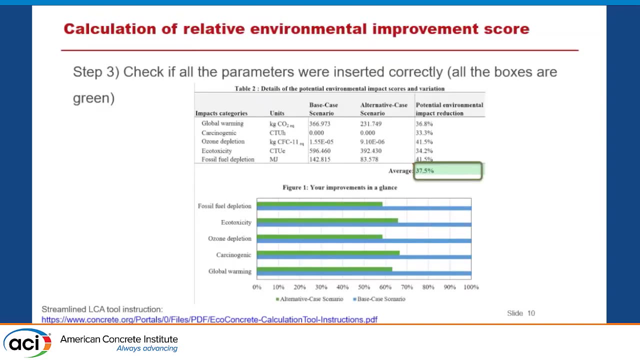 available SCMs, For example silicopium or fly ash, in some of the countries are not produced because they don't have any coal power plants and they have to import it from overseas. For the environmental impact calculations we not only focused on CO2, but we also consider other impact categories here- carcinogens. 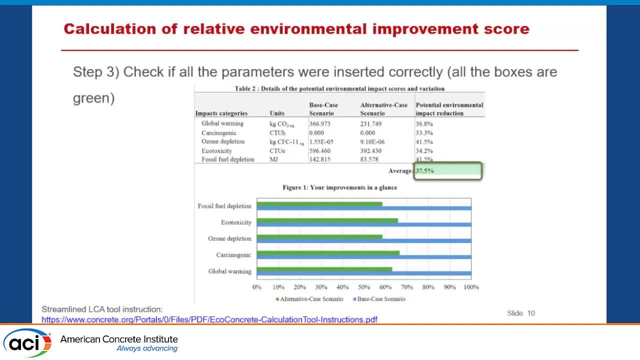 ozone depletion, ecotoxicity and fossil fuel depletion as five main important impact categories that will affect the life cycle, environmental impacts of the materials and the weighting system among these five different categories was like averaging the amount of reductions that we caused by introducing our new mixture For the gratings or scores of the materials that we are using. we are 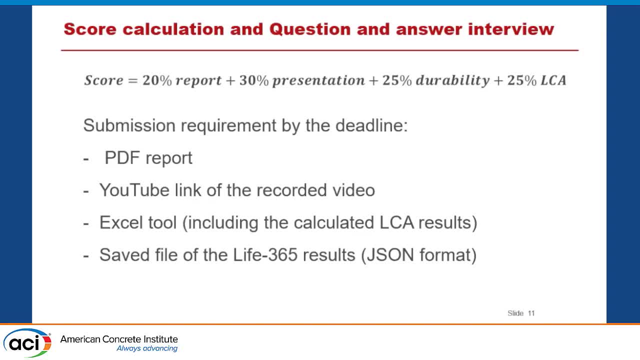 scoring. here we consider different weights, so we not only consider the amount of reductions that they observed in terms of the environmental impacts and the improvement in the durability, but we also try to work with them to improve their communications, because we realize that we may be able to develop. 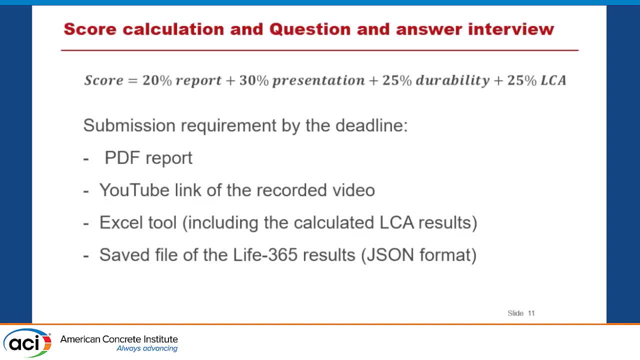 great mix design, but we need to communicate this with our appropriate audience in an effective way. So presentation and poster and interviews are two more important, you know components, and almost half of the scores in these competitions, in this competition, is assigned to this- these two important metrics. What did we learn from this competition? I forgot to mention. 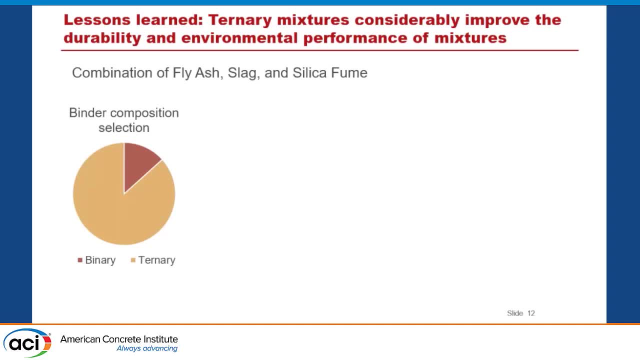 that we have held three versions of this competition. the first and the second versions were held in person at the ACI convention. so the participants brought their specimens here and we tested the electrical resistivity and compressive strength. but thanks to the COVID we went virtual and 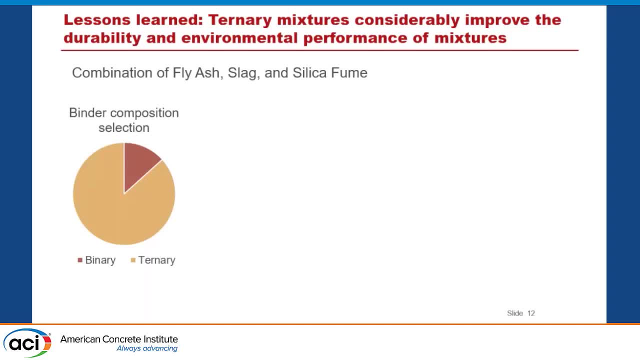 since then we are organizing this competition virtually, and the next version is going to happen after the New Orleans convention, spring 2024.. So these are the results of the last version happened in Atlanta Georgia convention And what we learned first of all is that students chose mostly ternary blended. 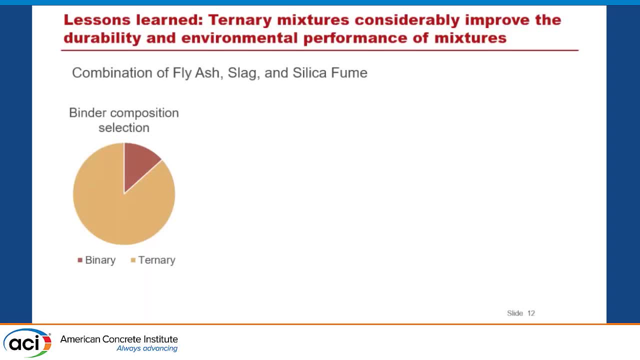 cements because they thought that gives the most out of the amount of constraints that you have in the mix design definition and it's a combination of fly ash, slag and silica fume and more than eighty percent of the. the teams chose ternary mixtures, But why? We saw that on average ternary mixtures. 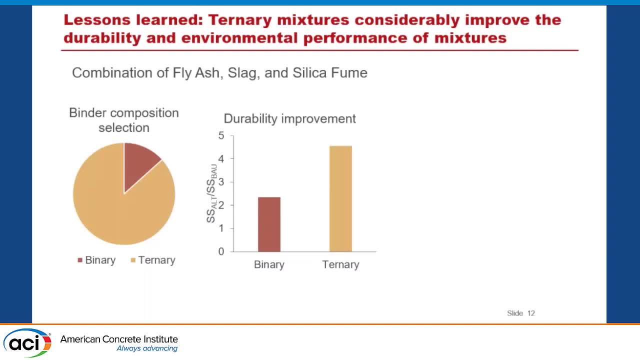 could improve the durability or the service life of the concrete by almost four folds, as opposed to binary mixtures that increase the durability by two folds. And the second metric: when we look at the environmental impacts, we saw that the amount of savings in terms of the average environmental impacts 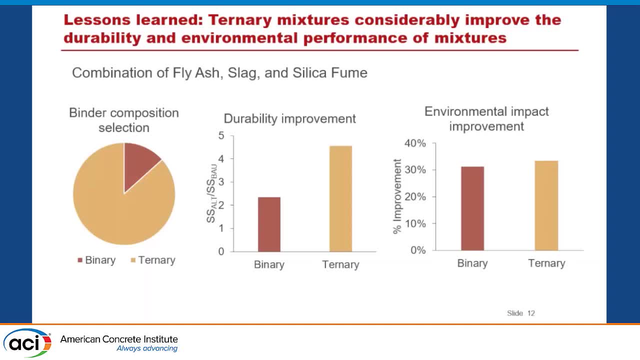 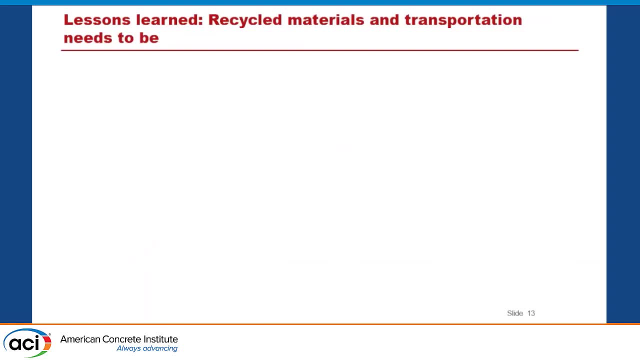 reduction was in ternary. blended cements was a slightly larger than the binary cements. How about the lifecycle perspective? We also learned that there are not some or enough clarifications in the rule and we had to emphasize on some important points that the student like generally. 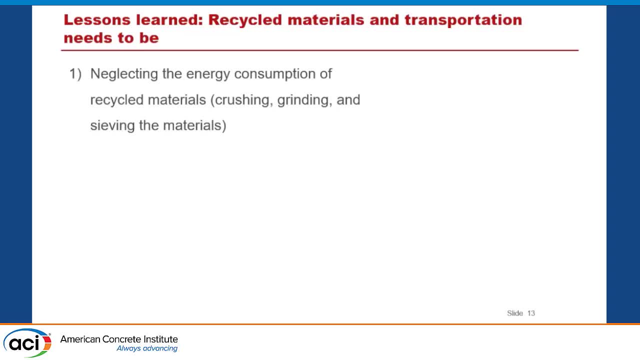 civil engineering students didn't consider, First of all, was the amount of energy consumptions associated with the processing of the recycled materials. So when it comes to recycling materials, notionally students consider that as a burden-free or zero emission material, So they didn't assign any. 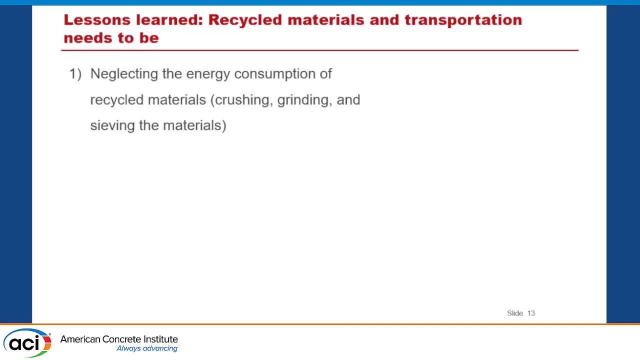 elements to the emmissions, But in reality we see that, for example, many of these materials need some post processing activities. slack means grinding, etc. So this is one point that we think and we emphasize in the new version of the competition in the rules as well. The second was again the 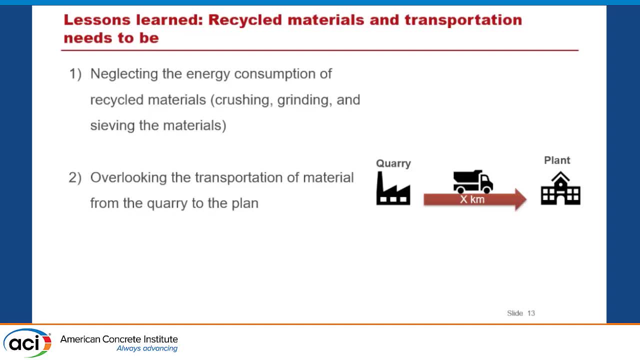 transportation. We mentioned that in the rules but we realized that the transportation of materials from Quarry to the university was usually neglected or was, partially neglected, removed, meaning that again from the distributor to the university, the transportation distance by truck was considered. but if it comes from 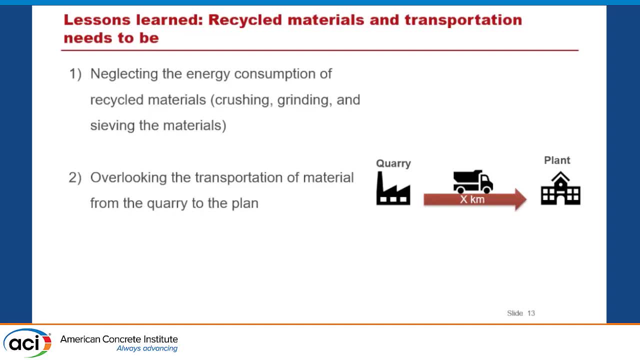 overseas or another country. the shipping wasn't considered in the environmental impact assessment. Lastly, not satisfying the minimum content of aggregates. We realized that when students consider recycled aggregates in their mix design and when they wanted to define an equivalent mix design when they considered the virgin material. 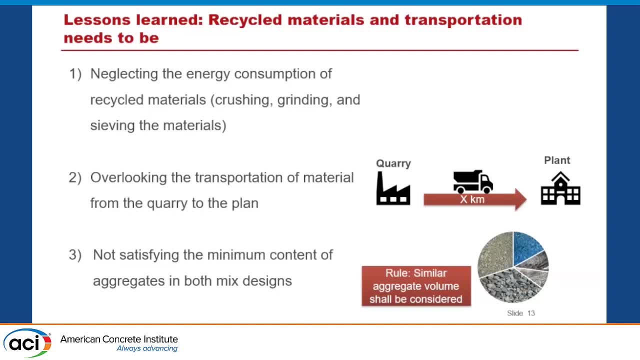 we know that the density of these materials are quite different from each other. When they designed this mixture and when they considered also a different density of binders, they didn't adjust the quantity of the aggregates and they considered them equal in terms of mass. 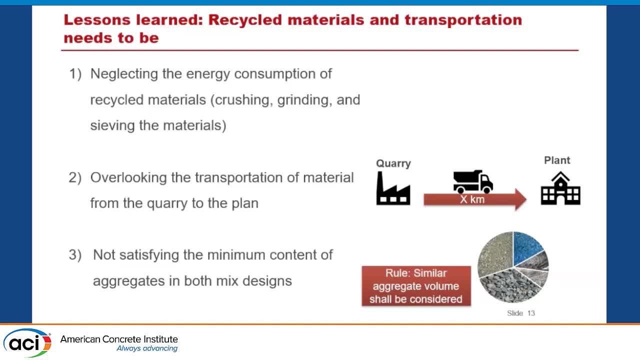 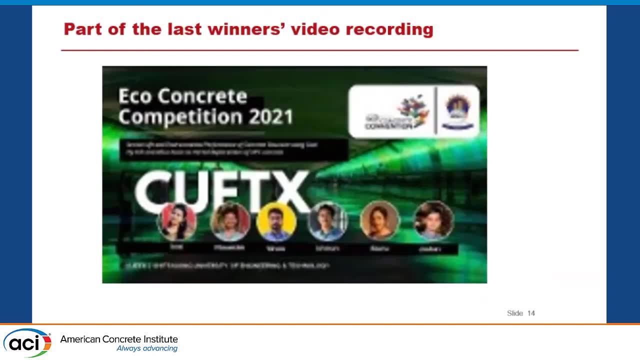 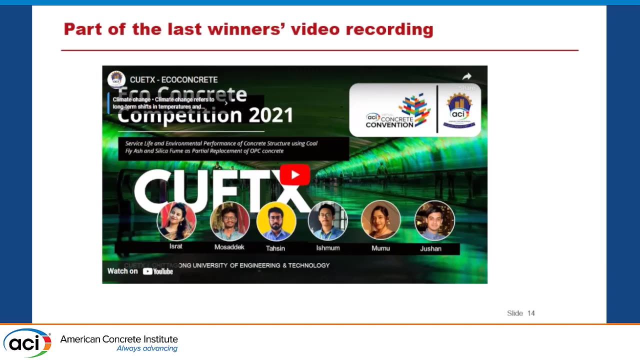 Again, we consider this as a penalty in the competition and we again emphasize that in the new version of the rules. Overall it was a great experience, particularly the last one that we held virtually, because it was sort of an equal access for all the students around. 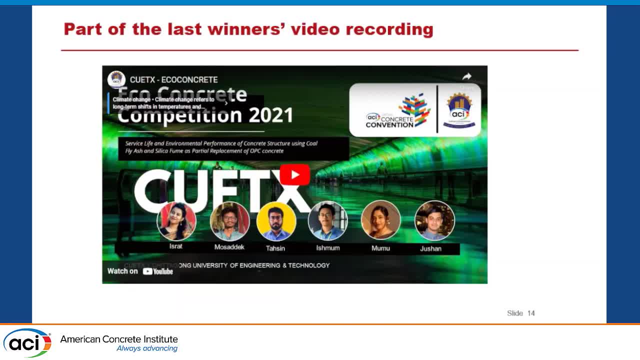 the world to participate in the competition and we had a lot of participants from different continents- Asia, Europe and, as usual, South America, Central America- and I'm just going to play the video that the winner of the last competition submitted and share the experience with you. 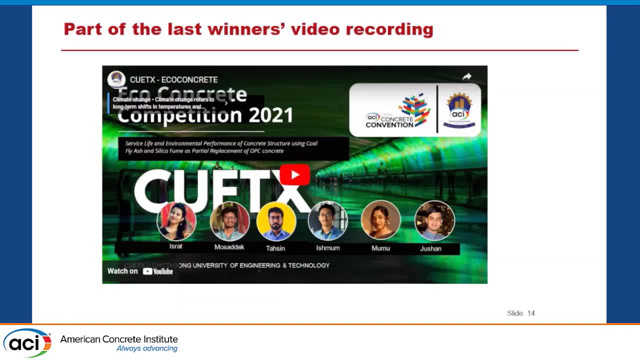 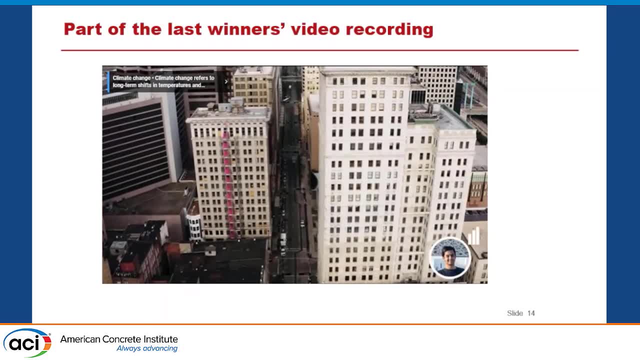 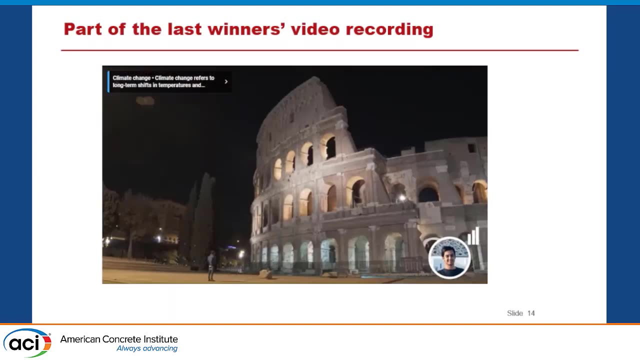 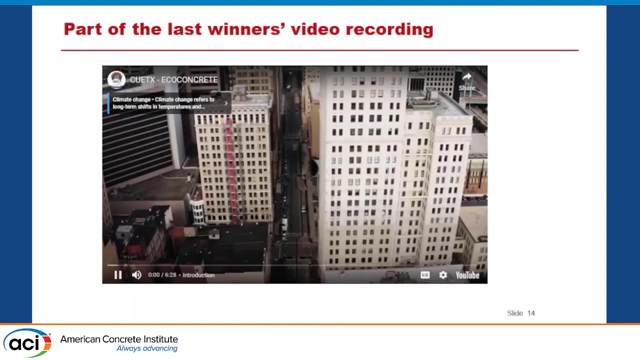 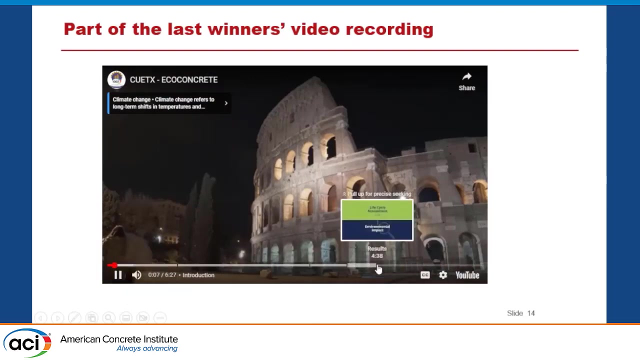 You guys, that's what: Concrete, one of the most widely used materials. somewhat, I'm sorry, I just want to go towards the end. The world has been used Concrete, one of the most widely used materials of the world, since the dawn of humanity. As we know, life cycle assessment helps us analyze. 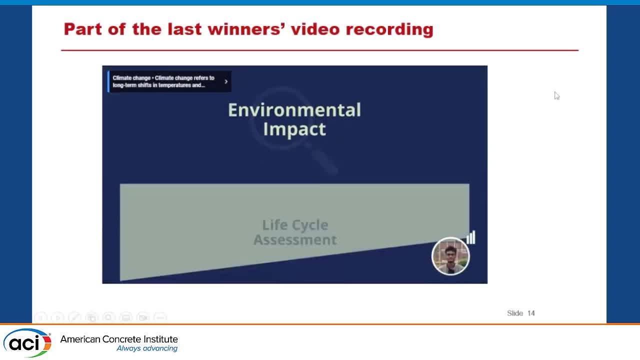 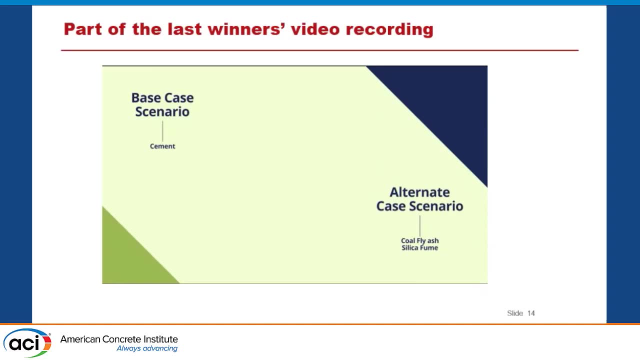 the environmental impact of a material's entire life cycle, which includes its extraction, production, transportation and distribution, and, after analyzing each material, we have found an average environmental impact reduction of 15.4 percent from the base case scenario to the alternate case scenario Individually. 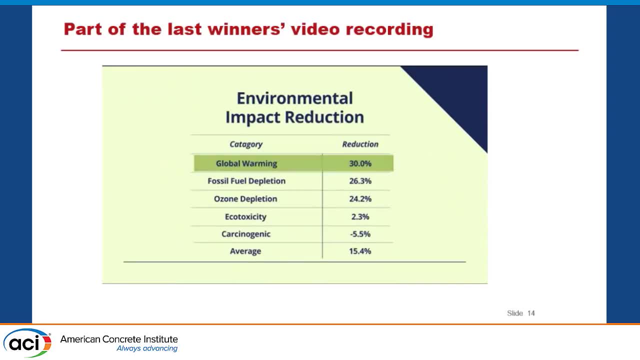 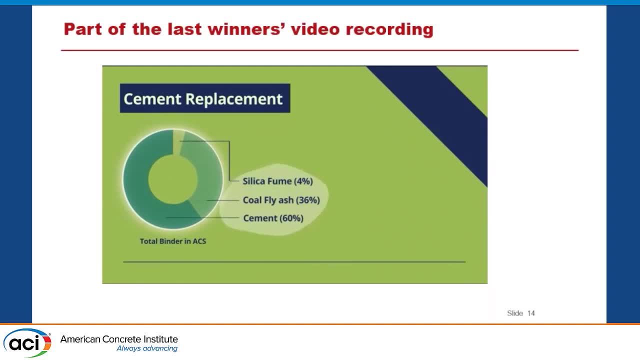 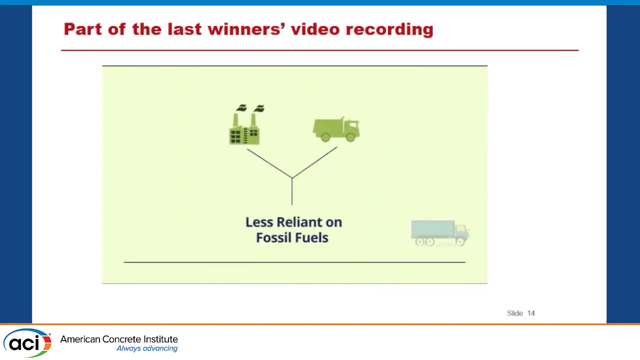 it shows, the highest amount of reduction is in global warming, followed by fossil fuel depletion and ozone depletion. The reduction has happened due to the partial depletion of coal, fly ash and silica film, as their production and transportation are less reliant on fossil fuels and emit significantly less. 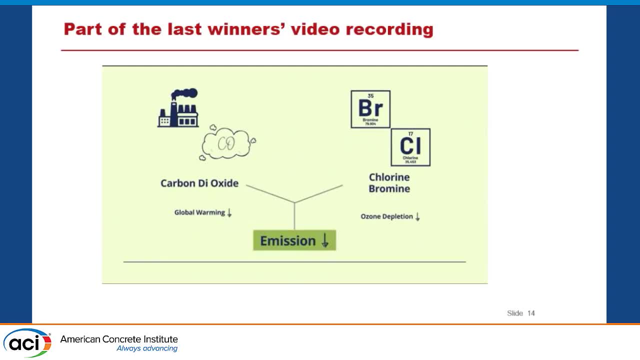 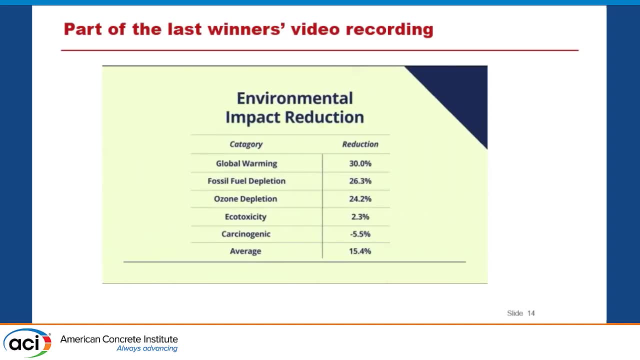 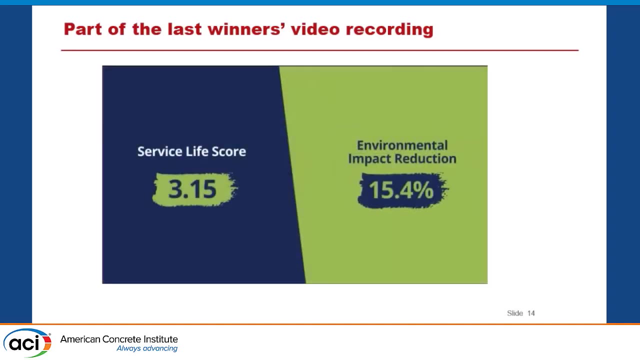 carbon dioxide or any other harmful gases like fluorine or bromine. However, silica film often has impurities like lead and copper, and this may lead to a comparatively less environmental reduction in ecotoxicity and carcinogenic impact, but these can be justified with a massive increase in 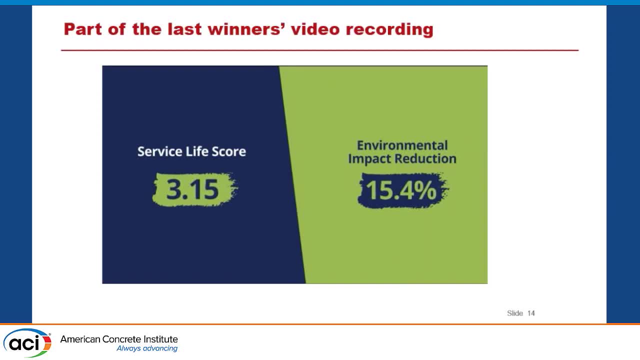 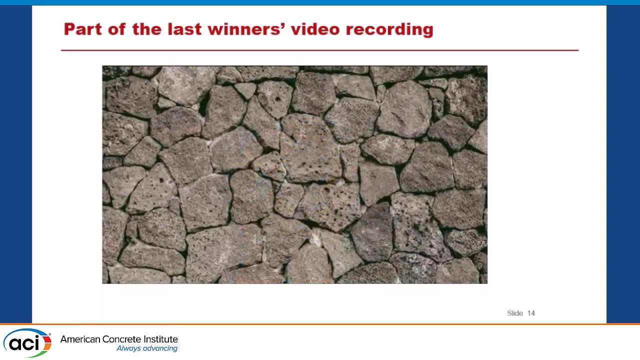 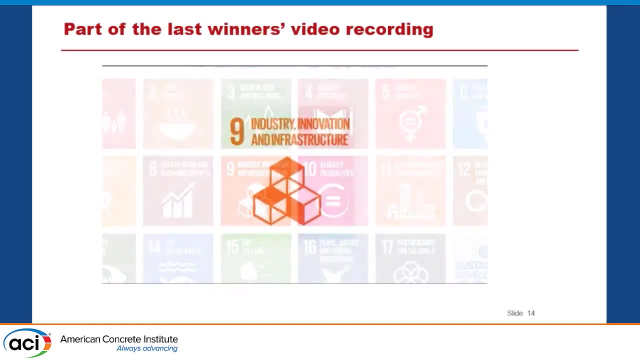 service life and a overall reduction of environmental impact. This mixed design tries to impact the least amount of environmental impact without compromising durability. Our project will bring us one step closer to achieve sustainable development goals. It will ensure a resilient infrastructure, resulting in a sustainable communities. it will utilize huge amounts of 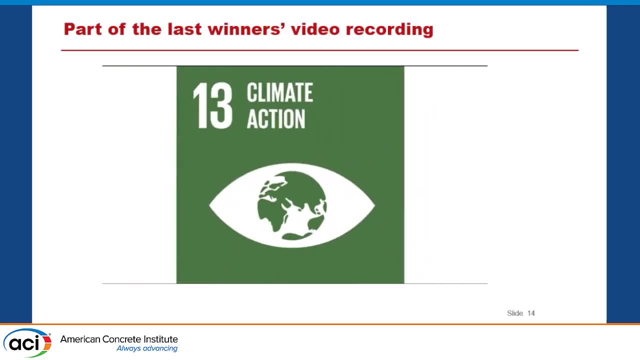 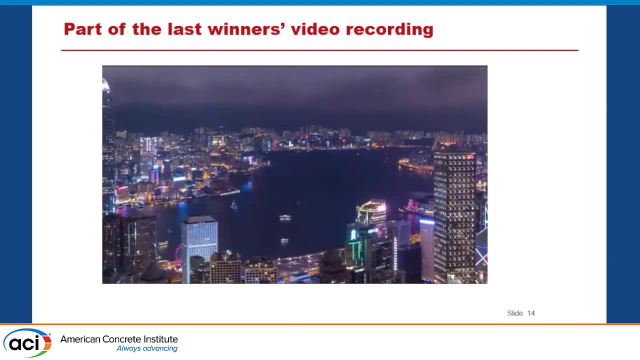 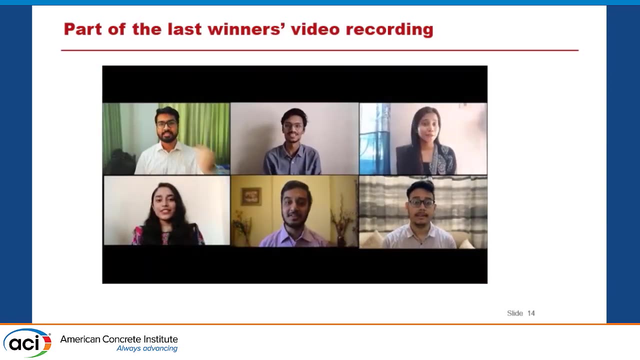 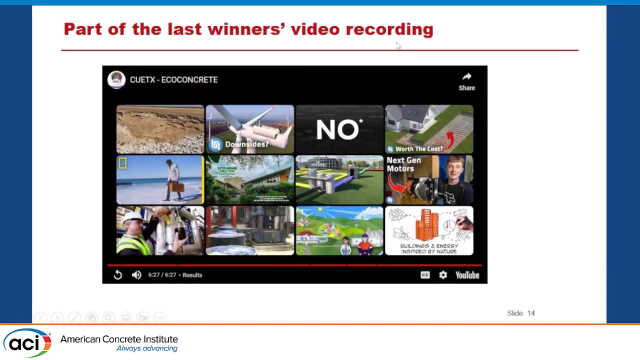 industrial by-products and, finally, by reducing global warming and other environmental effect. it will be bold action against climate change. it's time for taking innovative steps in construction for the betterment of planet earth. so you saw that there was a lot of cool editing and insights from 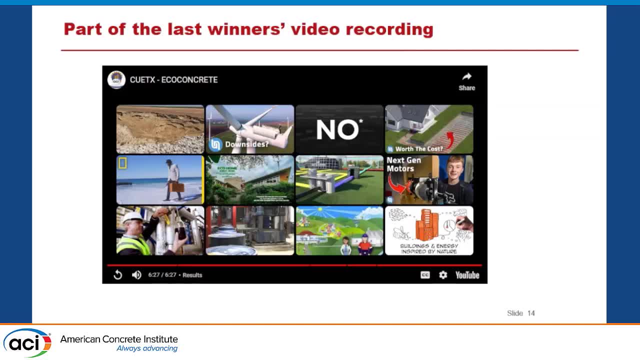 the students. we definitely asked the student to do to do a lot of trials and errors to find their optimizing issue and you saw that how silica film and fly ash ended up with the improvement in the environmental impacts and the durability of the mixtures. one thing that I should notice that last year I was working at the 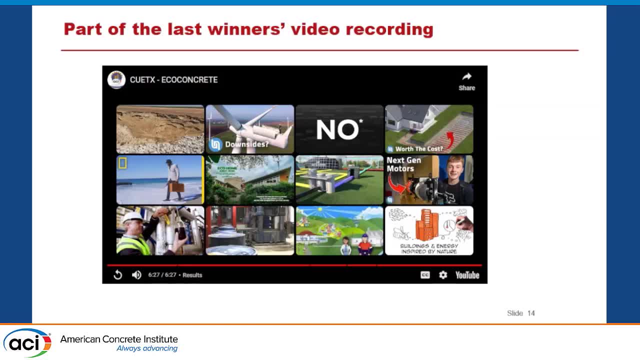 University of Michigan and I was teaching a course on sustainable infrastructure and I use this- the same format of the competition, but in terms of course projects. at the end I me for reduction of- although they were not bez였lutman students, i was at the school of environment and sustainability. 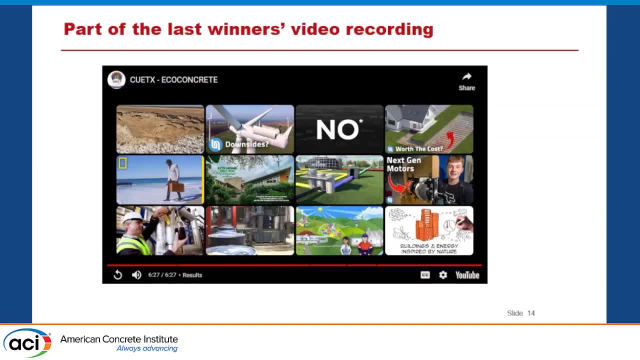 so I would recommend this: materials that are available on the both sides of rules, that the instruction about how to use the tool. they are all over there please use. feel free to use it in your course or in any other educational documents or sessions that you would like to organize in the future. lastly, all right, I have to. 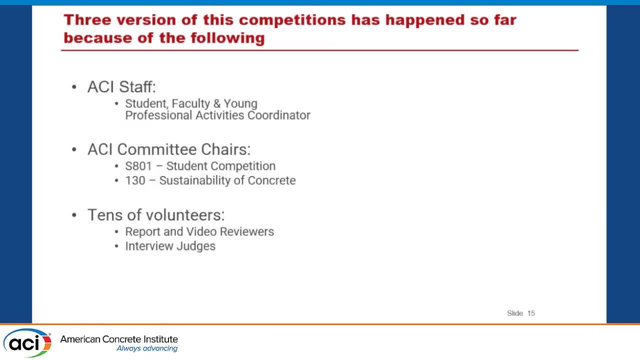 thank three different communities from ACI who have helped us a lot with this competition. this competition would have not happened without their help. first of all, key ACI staff, student, faculty and young professional activity coordinator, and also the competition coordinator, helped us a lot with you know.